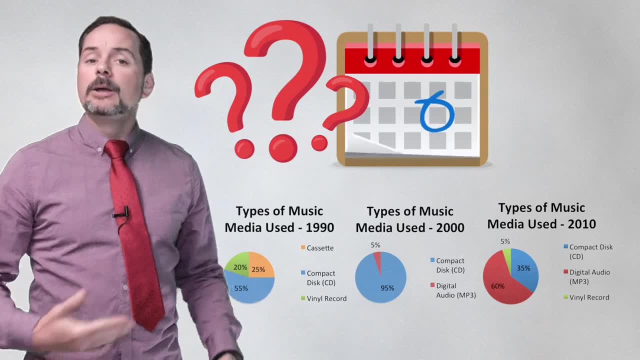 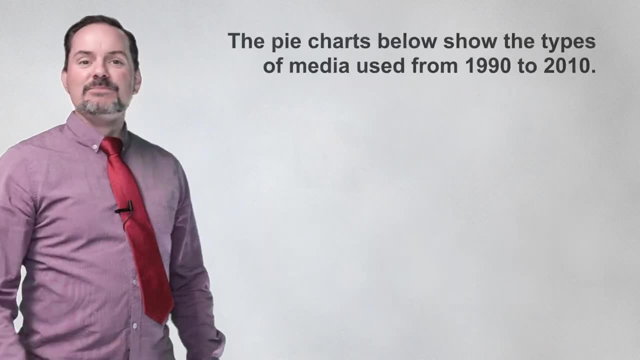 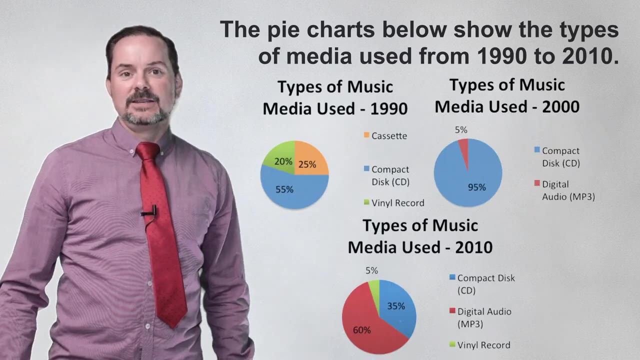 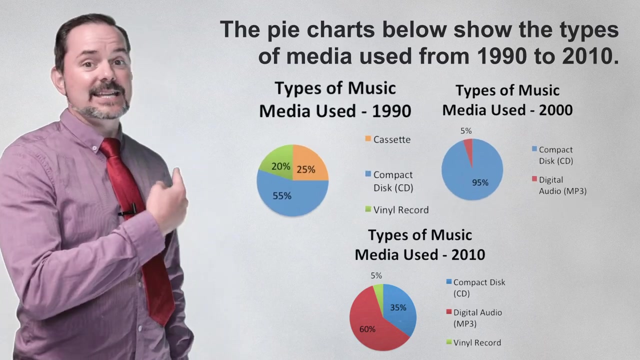 This is simply because we have no idea of the data between the time periods. Take the example of this question answered by the student regarding music media. We have three time periods: 1990, 2000, and 2010.. Now we can definitely see that more people listened to CDs in 2000 than in 1990.. 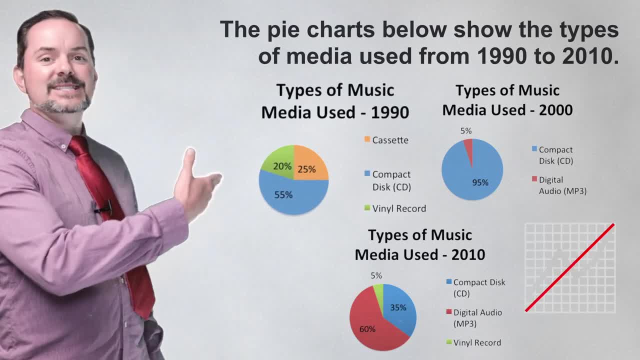 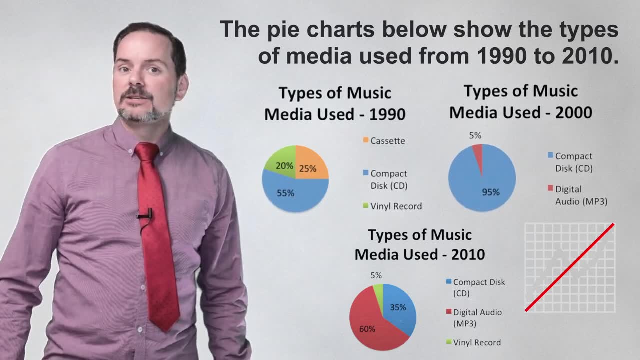 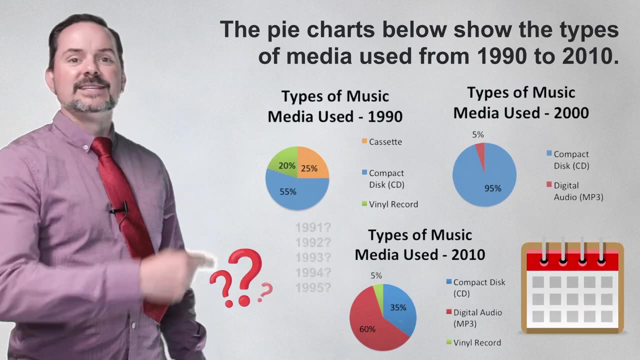 And it's easy to assume that there was an increasing number of people listening to CDs between 1990 and 2000.. However, this could be a wrong assumption. We don't know the information for the years between 1990 and 2000.. 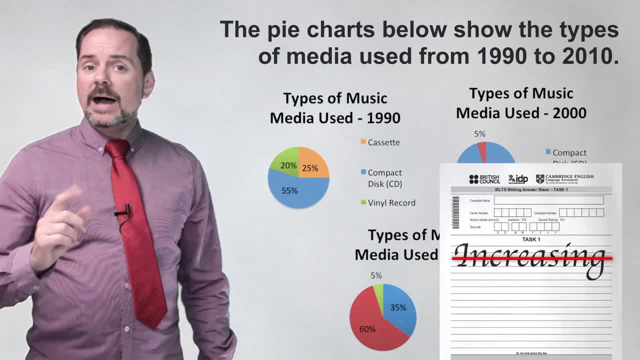 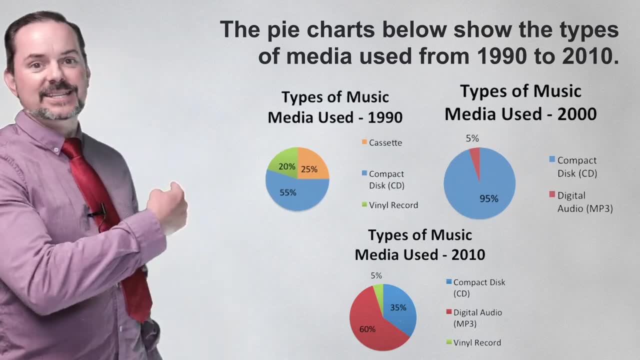 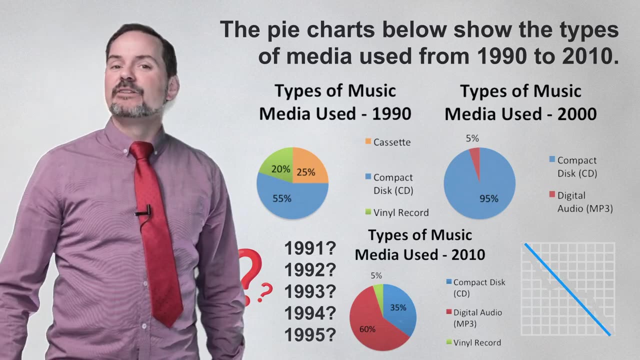 Therefore, it is inaccurate to say that, While it's true that the number of people using CDs had increased in 2000 compared to 1990, we don't know what happened in 1995.. There might have been a decrease in the number of people listening to music on CDs. 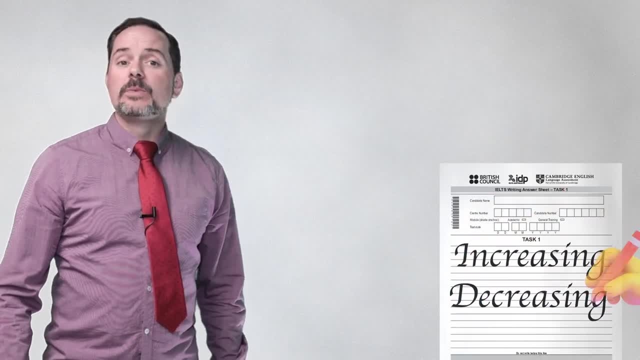 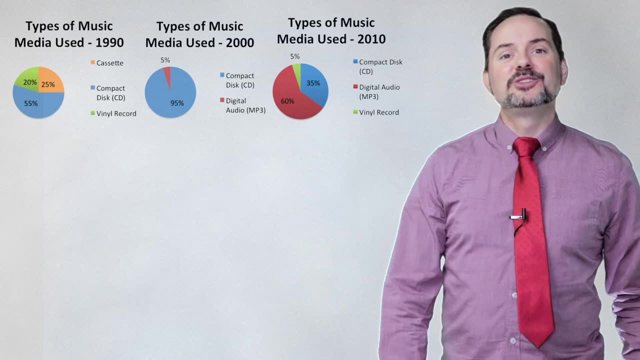 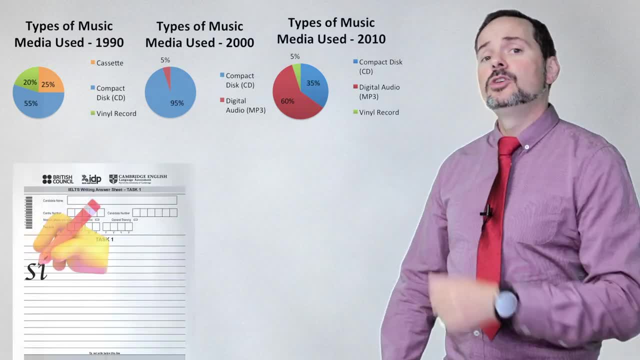 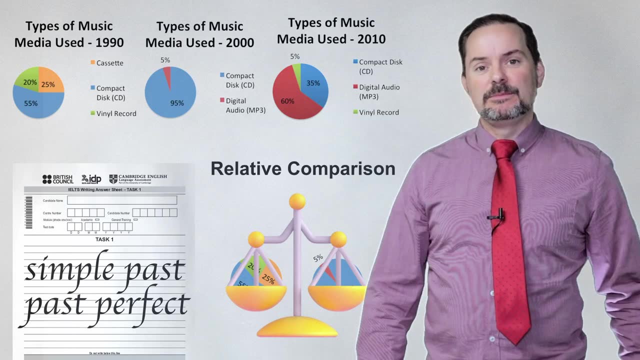 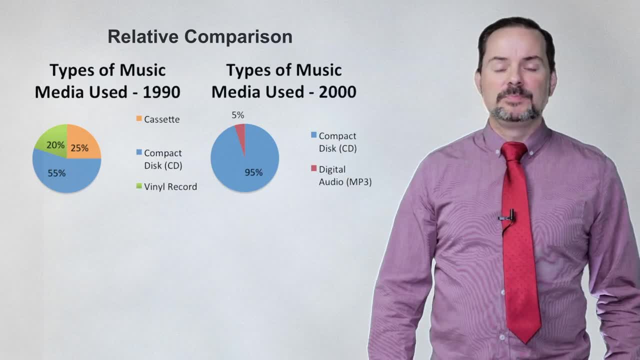 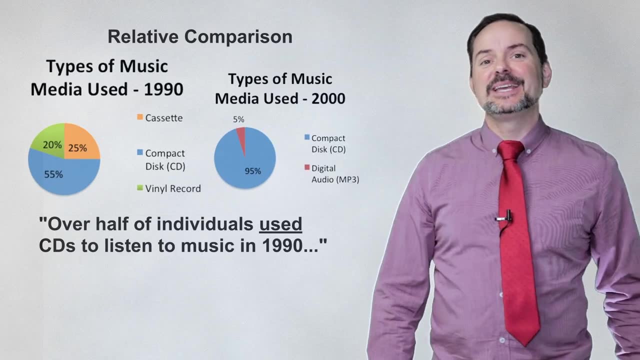 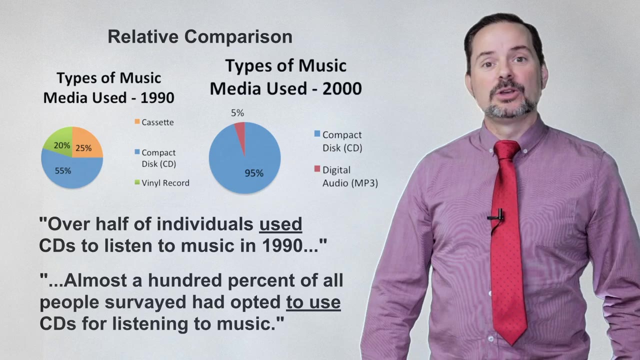 Take, for example, the CDs in 1990 and 2000.. It's best to state that just over half of all individuals used CDs to listen to music in 1990.. However, by 2000,, ten years later, almost a hundred percent of all people. 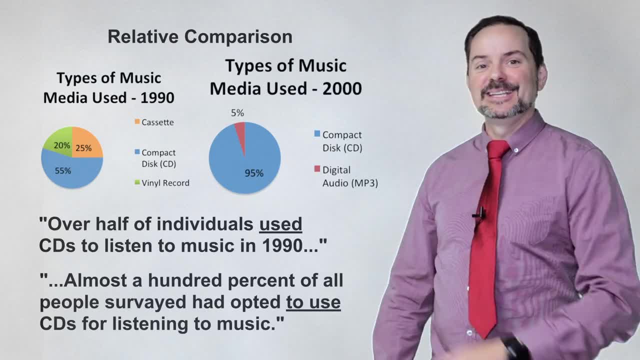 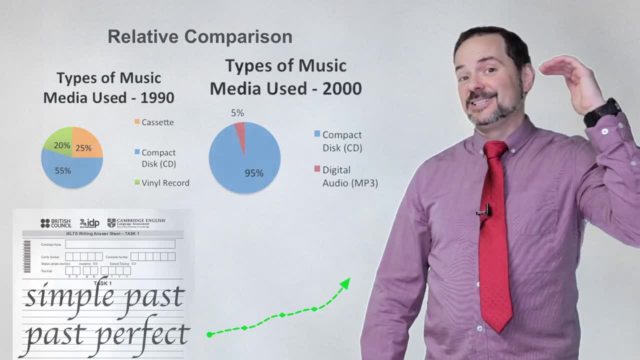 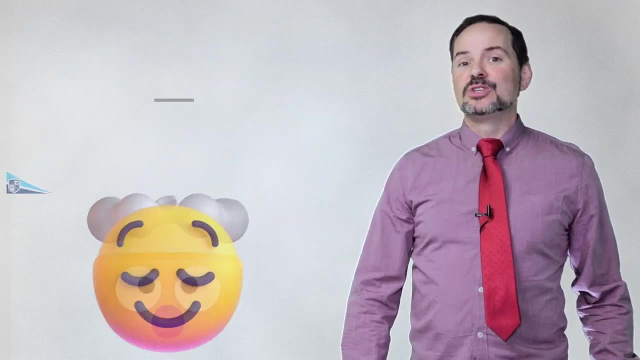 surveyed had opted to use CDs for listening to music. It's this kind of simple past and past perfect that will be accurate and get you those high scores. To understand the basic concepts of graphs and charts, make sure to use your interactive course in your premium package at aehelpcom. 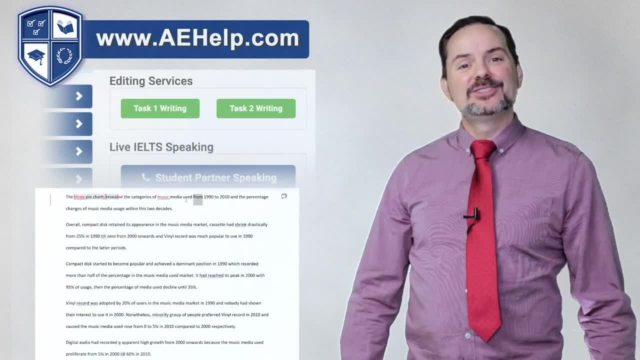 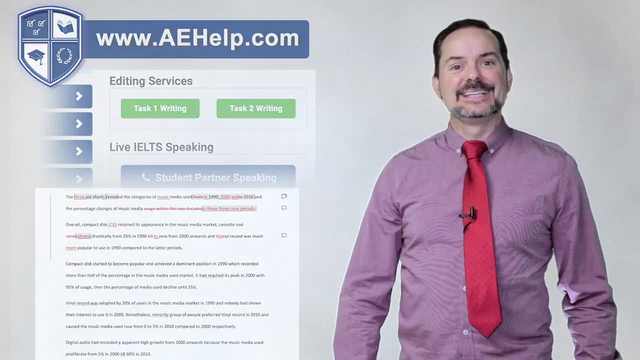 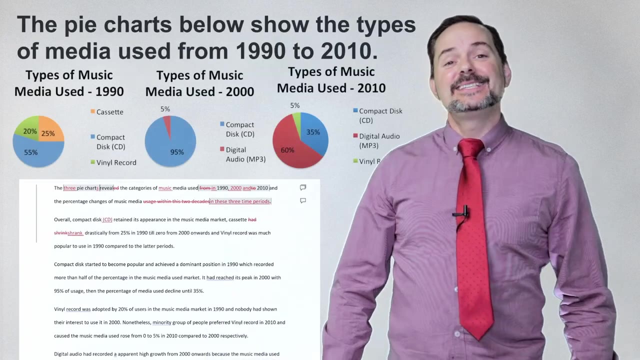 Once you're ready, use the task one and task two editing services for feedback and correction, just to make sure that you get the most out of it, Make sure that you really have the right idea for your next exam. Now let's take a look at this student's task one submission for this question to see how. 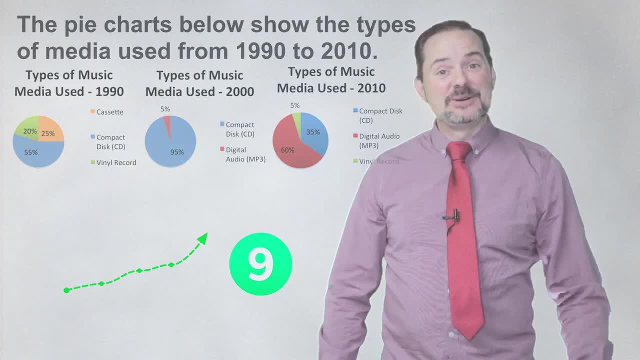 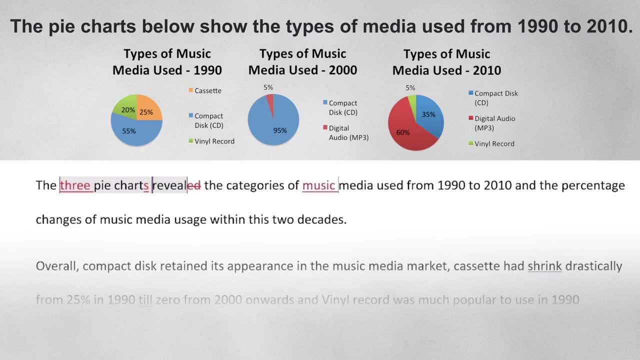 he can improve from a band six to a band nine. response: When we look at the introductory paragraph, the three pie charts reveal the categories of music media used in 1990,, 2000, and 2010, and the percentage changes of music media. 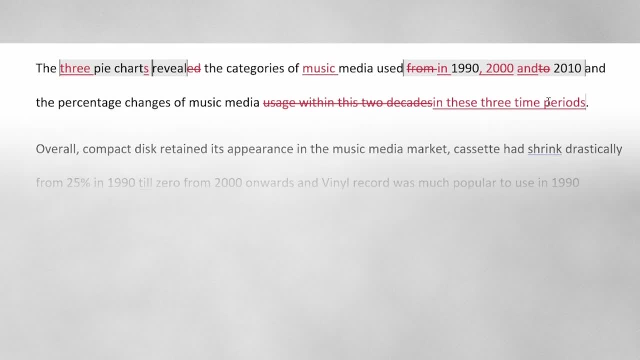 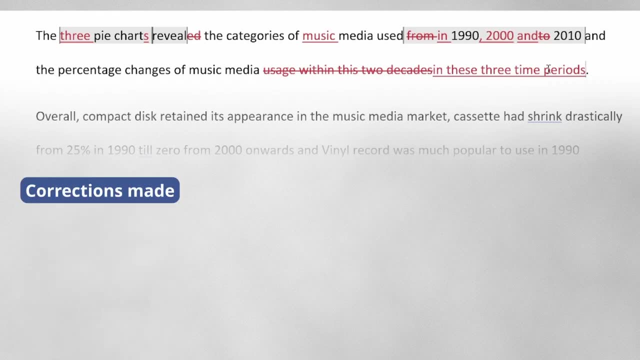 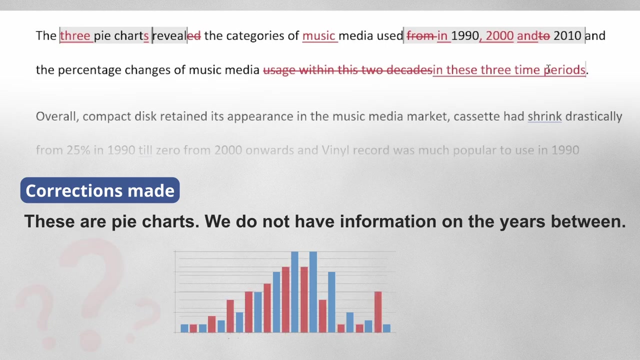 in these three time periods. Notice the corrections. The student wrote media used from 1990 to 2010.. This is an incorrect format again, because this is not a line graph. We do not have data for all of those years. 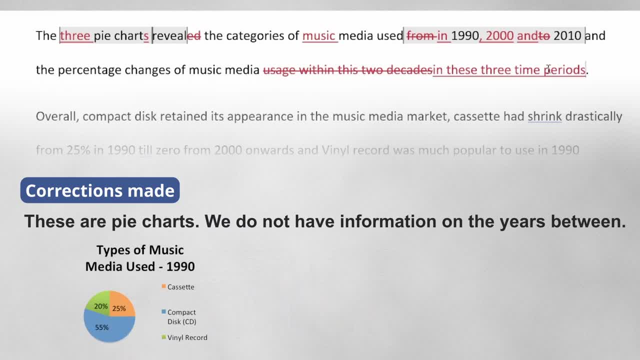 We simply have data for three time periods: 1990, 2000, and 2010.. Again, at the end of the introductory paragraph, notice the correction to usage with music Usage within these two decades. Once again, this is incorrect to state because we do not have the data for all of the years. 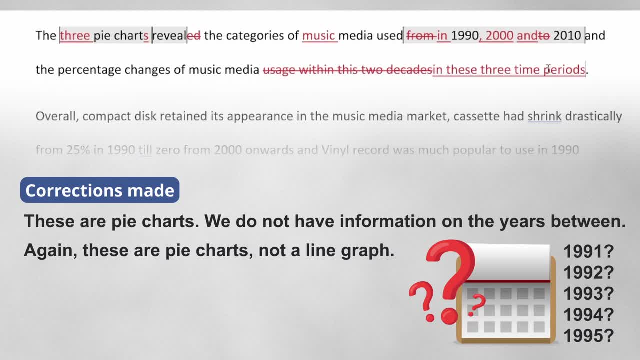 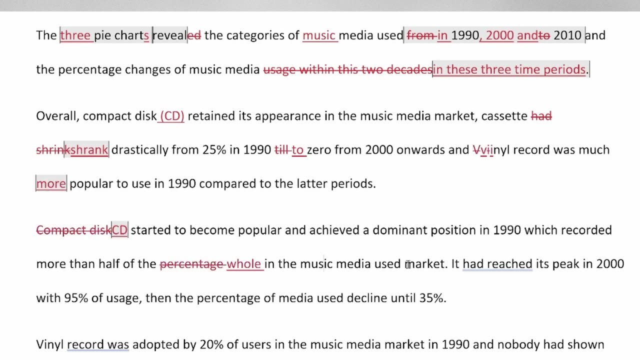 within these 30 years. Keep in mind you are writing for a pie chart, not a line graph. This is a major coherence mistake in this case and significantly drops scores. Following some corrections to content, grammar and punctuation: again, this candidate makes. 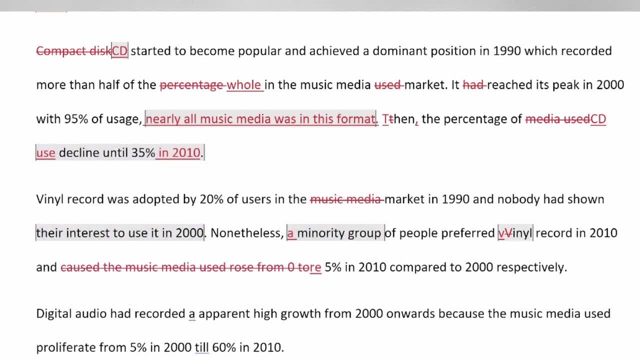 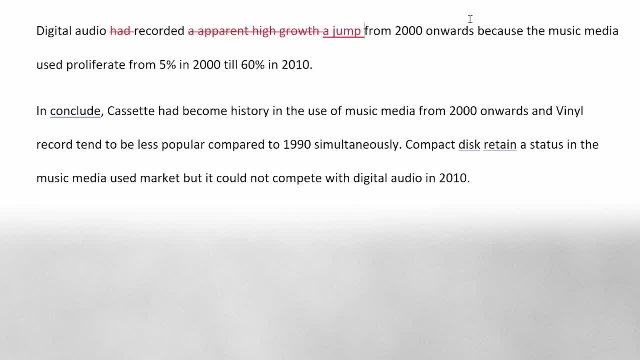 the mistake. This is an incorrect way of writing, as if this were a line graph rather than a pie chart, stating digital audio had recorded an apparent high growth from 2000, at 5% to 60% in 2010.. 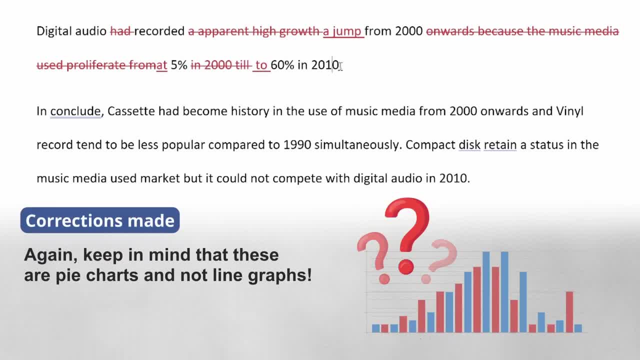 Since we do not have continuity, this needs to be adjusted. Digital audio recorded a jump from 2000 at 5% to 60% in 2010.. Make sure to pay attention to this kind of a mistake. Make sure to keep in mind that you are writing for a pie chart and not a line graph. 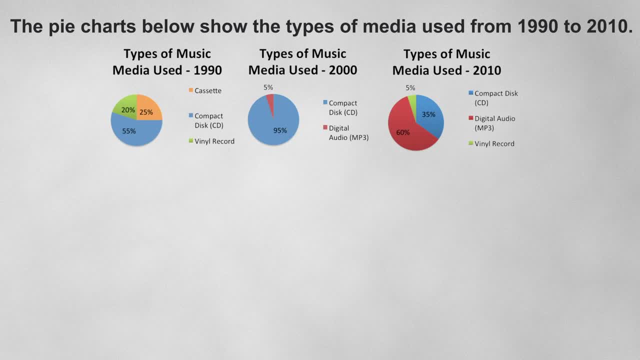 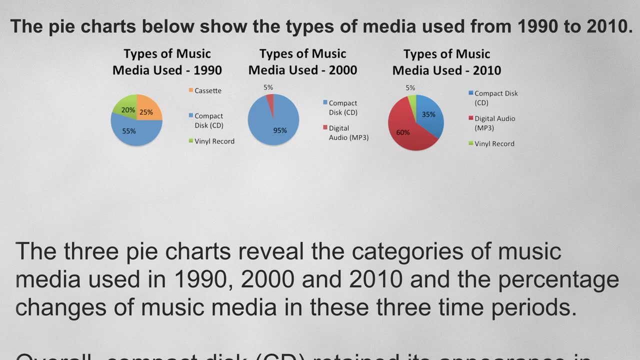 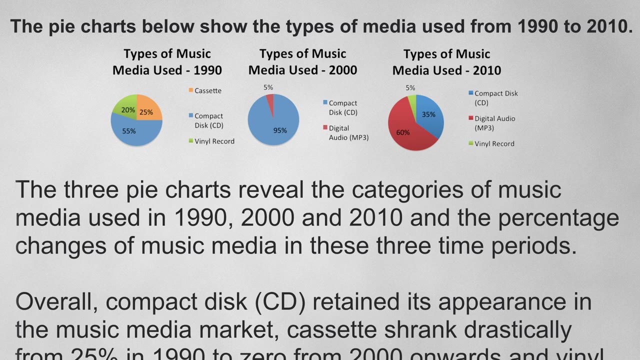 Know the difference, Let's take a look at the correct completed band 9 essay. The three pie charts reveal the categories of music media used in 1990,, 2000, and 2010, and the percentage changes of music media in these three time periods. 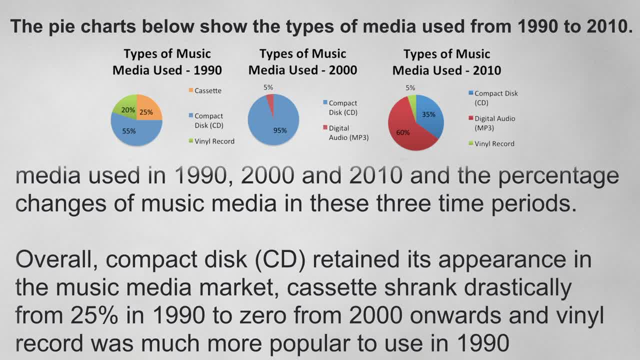 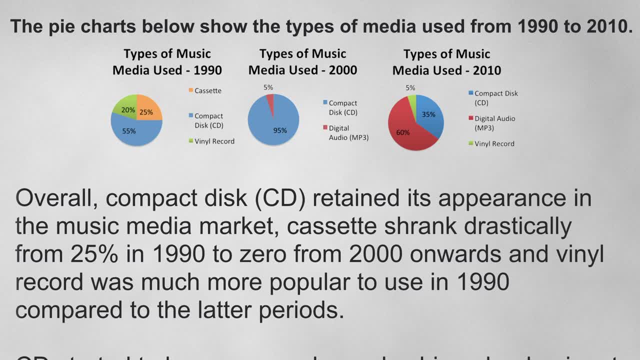 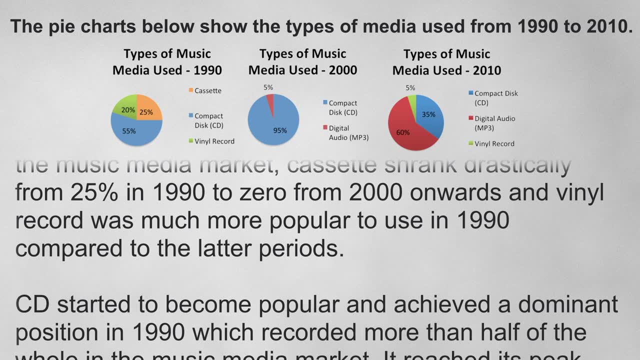 Overall. compact disc retained its appearance in the music media chart media market. Cassette shrank drastically from 25% in 1990 to 0 from 2000 onwards and vinyl record was much more popular to use in 1990 compared to the latter periods. CD started to become popular. 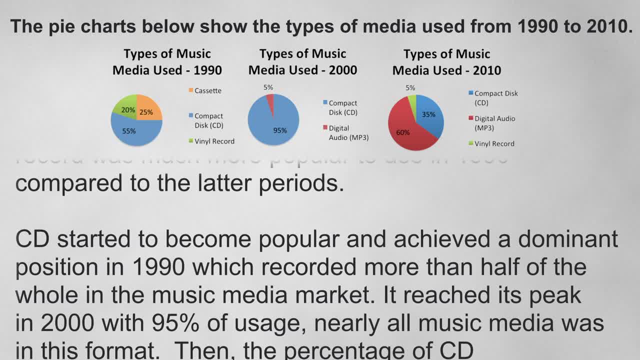 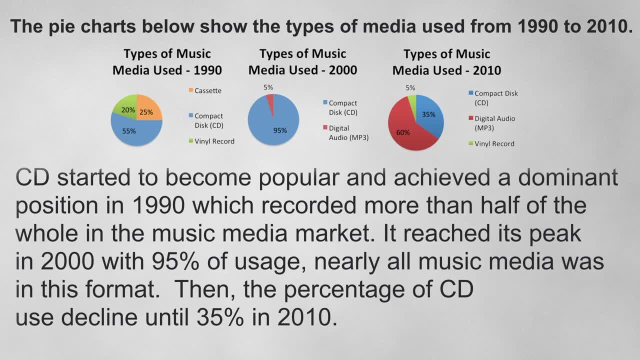 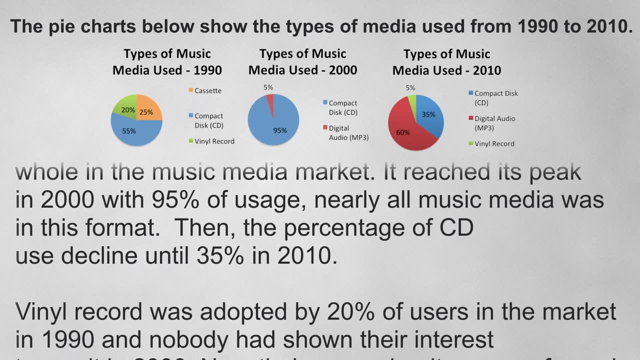 and achieved a dominant position in 1990, which recorded more than half of the whole in the music media market. It reached its peak in 2000 with 95% of usage. Nearly all music media was in this format. Then the percentage of CD use declined until 35% in 2010.. Vinyl record was adopted by 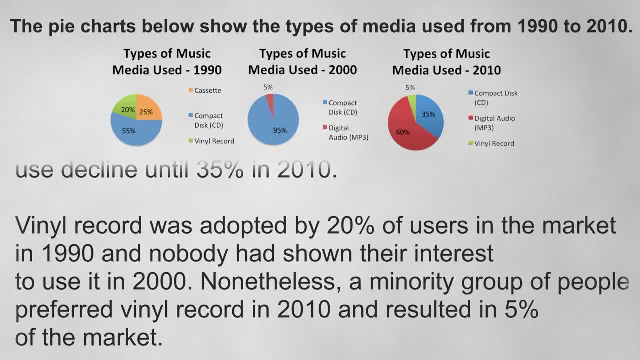 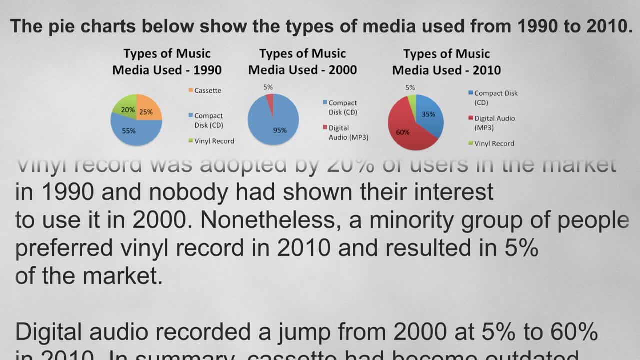 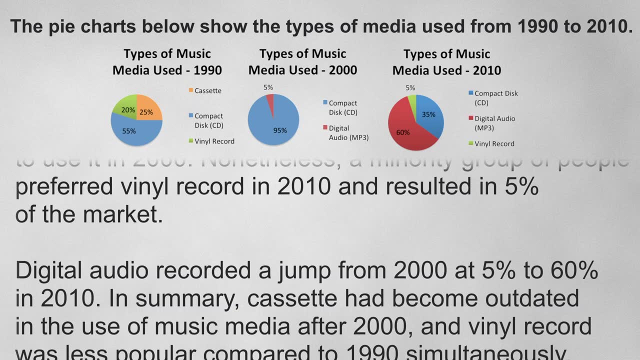 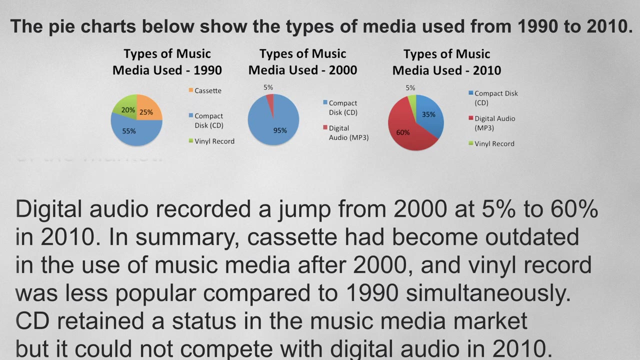 20% of users in the market in 1990, and nobody had shown their interest to use it in 2000.. Nonetheless, a minority group of people preferred vinyl record in 2000.. In 2010,, digital audio recorded a jump from 2000 at 5% to 60% in 2010.. In summary, cassette had 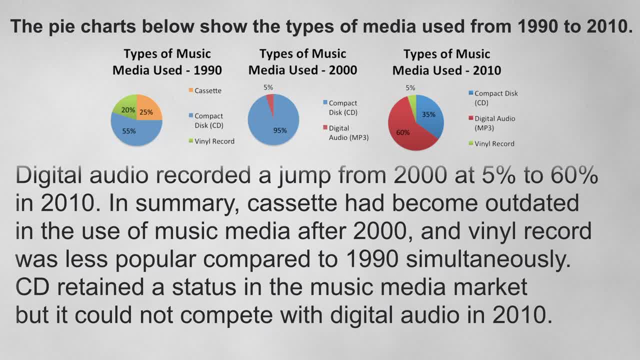 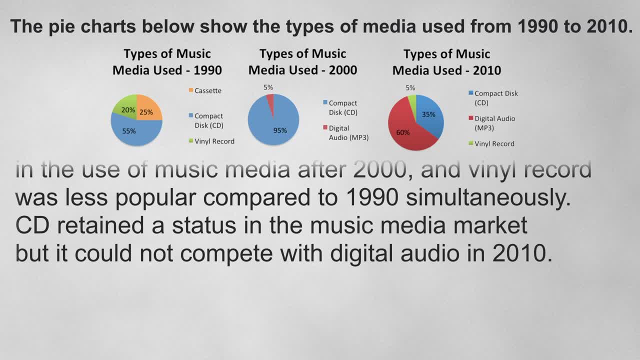 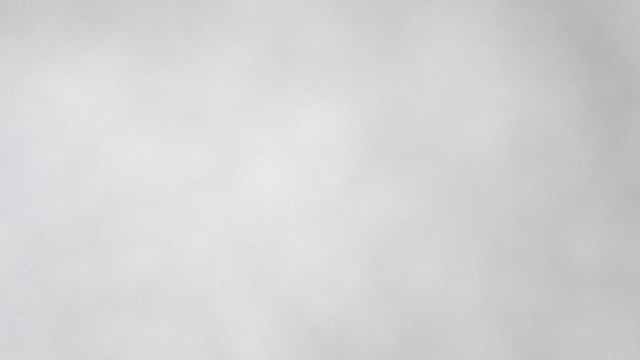 become outdated in the use of music media after 2000,. and vinyl record was less popular compared to 1990. simultaneously, CD retained a status in the music media market, but it could not compete with digital audio in 2010.. For the record, it was a very popular record. 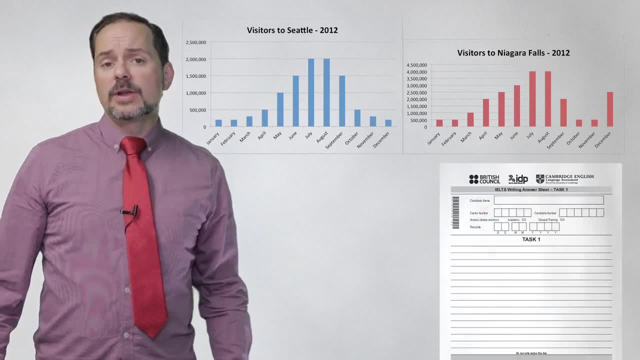 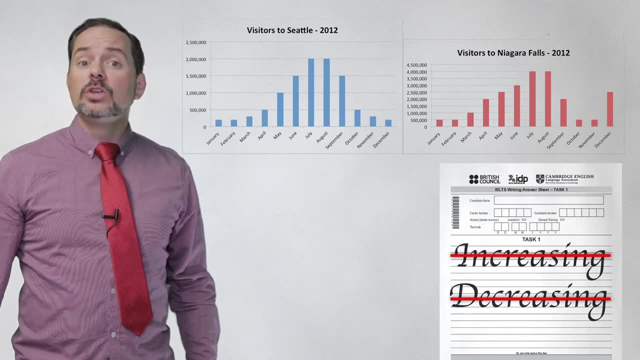 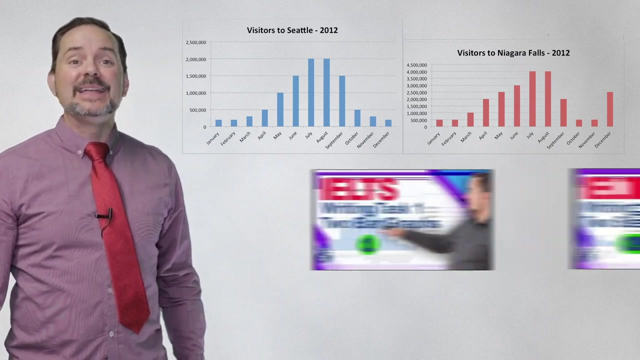 For bar charts, like with pie charts, using the progressive form, ING increasing and decreasing- is not always accurate. You have to be careful. You have to look at the data presented and make the right decision. To do so, check out the video at the end of this lesson that describes a perfect 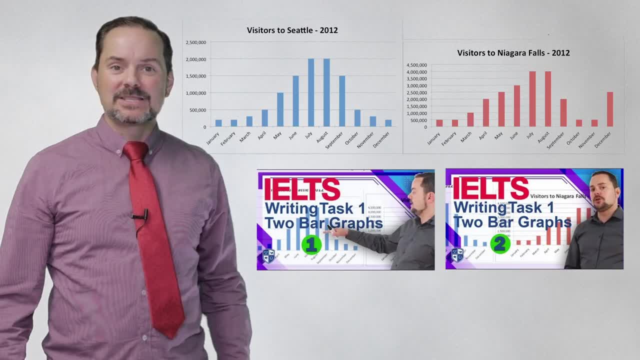 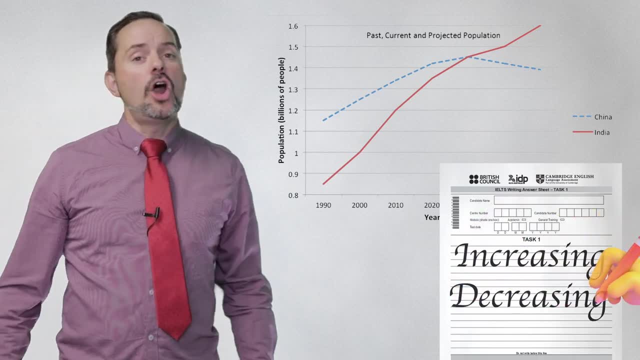 band 9 essay. when comparing two bar graphs, Also keep in mind that even for line graphs, the words increase and decrease are not always accurate. So if you have a bar chart that is increasing and decreasing are overused, So you should use synonyms to improve your lexical.